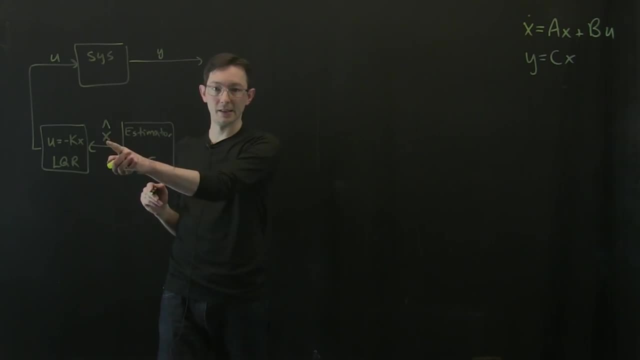 optimal estimator will estimate the state, So x. hat is an estimate of the full state x and it takes into account measurements y and also measurements of what the control is doing. u Okay, and so what we've shown in the previous few lectures, this is called optimal control. 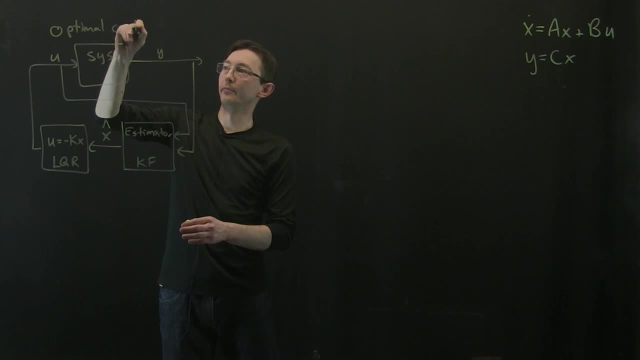 This, essentially, LQR is an optimal regulator. the Kalman filter is an optimal estimator. When you put these together, this is called LQG, or linear quadratic Gaussian regulator, And regulator just means that we're trying to drive the state of the system x to 0 to the origin. 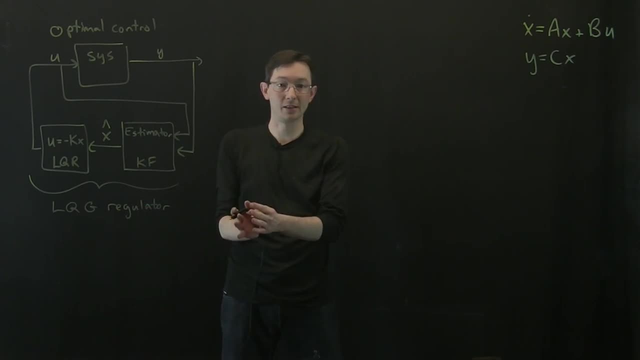 I could make this a reference tracking problem where I try to drive the state of the system x to some vector direction x. But if we're stabilizing the system, it's a regulator and what we've shown is that if the system is controllable, so if a and b are controllable and if a and c are observable- 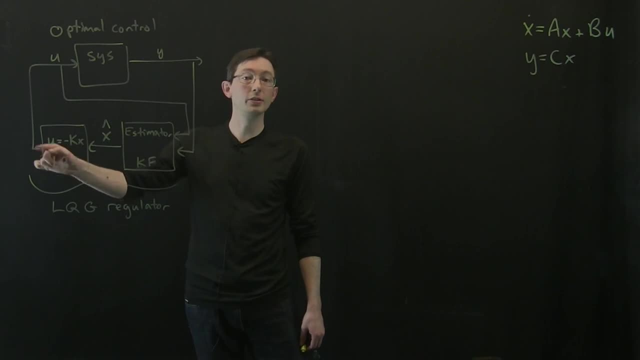 then it's possible to design this LQR regulator so that the closed loop eigenvalues are arbitrarily stable and it's possible to design this estimator block so that the estimate x hat converges to the true state x as fast as we want And there are some optimal eigenvalues. 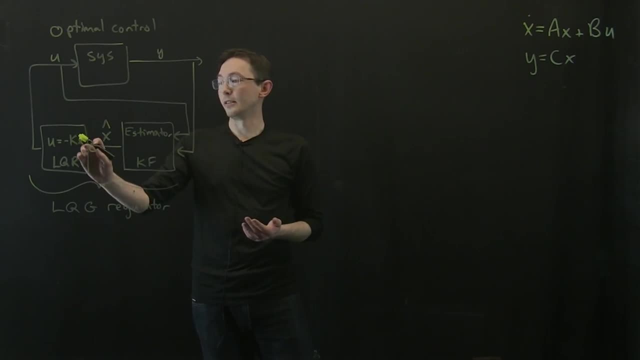 And there are some optimal eigenvalues based on trade-offs between accuracy of how fast you're tracking the state to 0 and how much control you're spending, and also a balance between the types of noises and disturbances you see in your system, And so this, broadly speaking, is the field of optimal control. 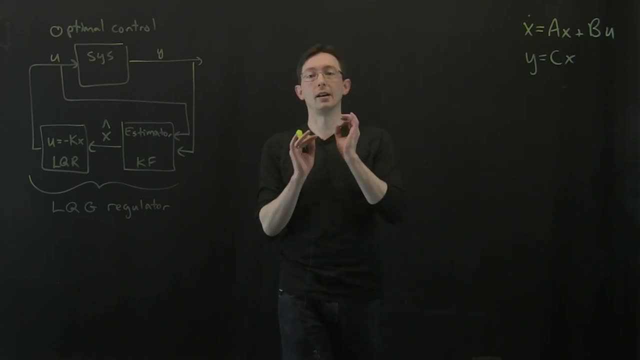 But today we're going to start talking about a very, very important modern perspective and control theory called robust control. Okay, So Well, robust control has been a mainstay and is still possibly the most used state-space formulation of control today. So if you have a state-space system, x, dot equals ax plus bu, y equals cx. chances are. 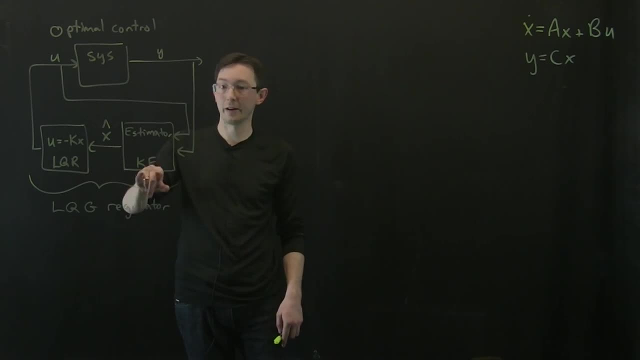 you're going to start by developing a LQR regulator and a Kalman filter, But there was a remarkable paper by John Doyle. So Doyle, in 1978, wrote this amazing paper, One of the most important papers in control theory ever written and one of my favorite. 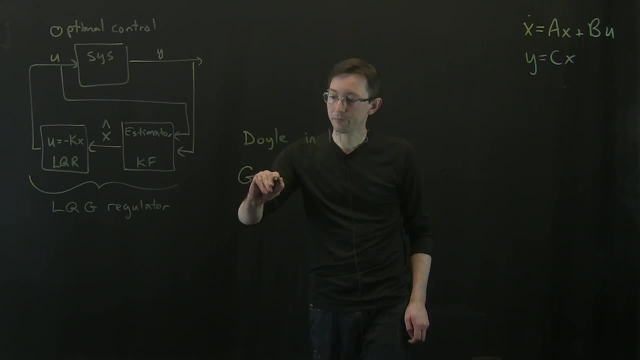 papers called Guaranteed Margins, And this means stability margins, Guaranteed Stability Margins for LQG Regulators. Okay, And I want to break this down for you. Okay, So, Guaranteed Margins for LQG Regulators. This is the title of John Doyle's 1978 paper. 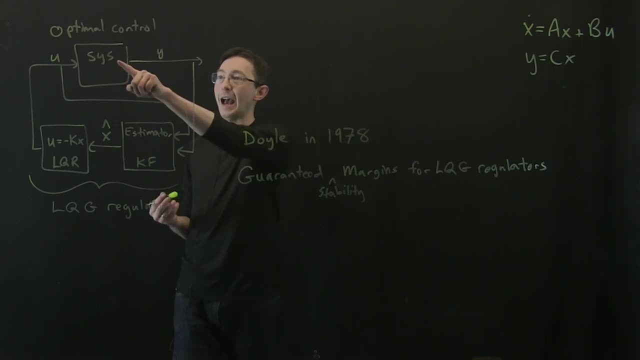 And it was well known at the time that if you actually were measuring the full state, if y equaled x and I didn't have to do a Kalman filter, then the LQR regulator was pretty robust. If I had some uncertainties in my system, if my system was a little bit different or 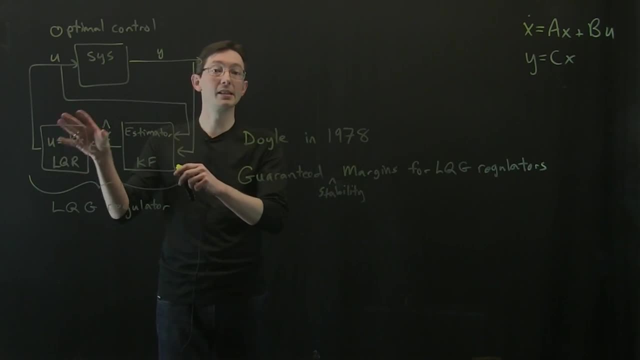 I had some time delays in my system. the LQR regulator would still be able to stop Okay And stabilize the system as long as y equaled x. Now what John Doyle was investigating in this 1978 paper is, if I don't have measurements, 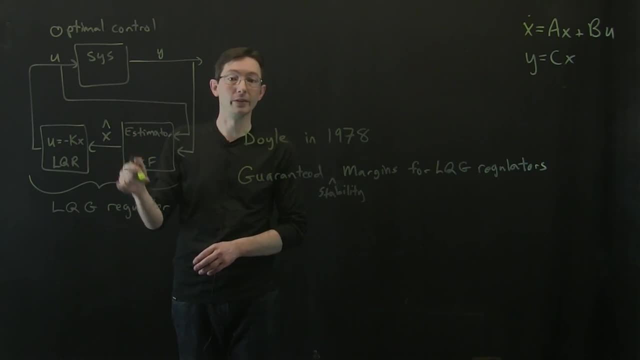 of x, but I have to build up an estimate using something like a Kalman filter. is this combined LQG regulator still robust to things like uncertainties in my system or time delays? And so, in this paper, one of my favorite things about this is the abstract. 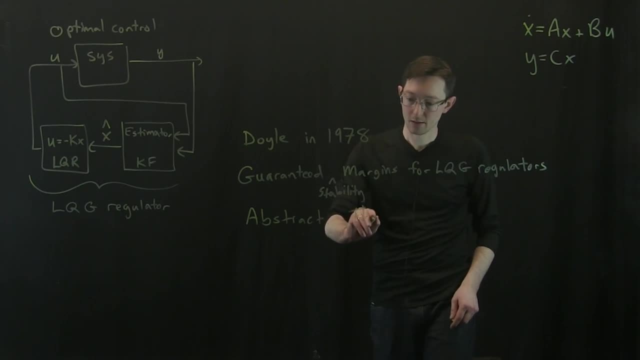 There ain't none. Well, I think the editor probably made him change it to: there are none, One of the simplest and most direct abstracts there in the literature. Okay, So what John Doyle showed in his 1978 paper is that there are no guaranteed stability. 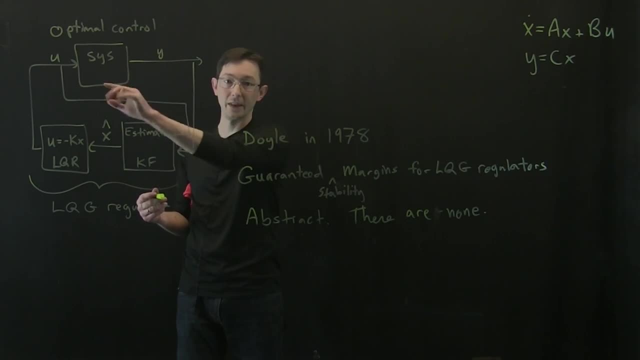 margins for LQG regulators. So, depending on my system and the types of noise and disturbances that I have in my system, there are no guaranteed stability margins for LQG regulators. So, depending on my system and the types of noise and disturbances that I have in my system, 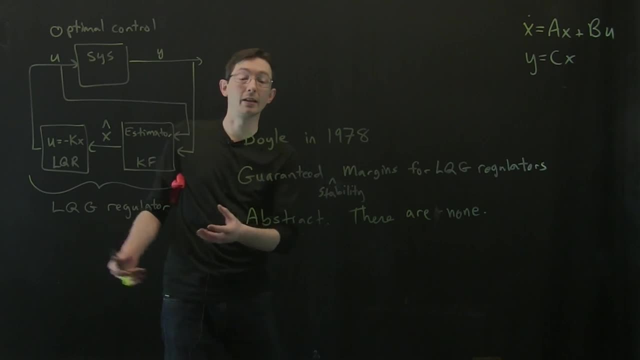 my combined LQR and Kalman filter. my LQG regulator might be arbitrarily sensitive to things like model uncertainty and time delays. It could be arbitrarily non-robust. Okay, This is really a beautiful paper. It's less than one printed page and it changed the field of control forever. 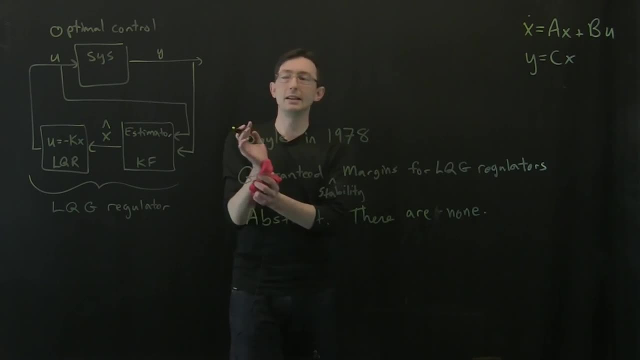 Okay, So instead. so there's this idea that we could change the eigenvalues of this LQR regulator. we can change the eigenvalues of this estimator to be whatever we want: to be: more stable or less stable. Okay, So this LQR regulator can change the eigenvalues of the closed loop system and this Kalman filter. 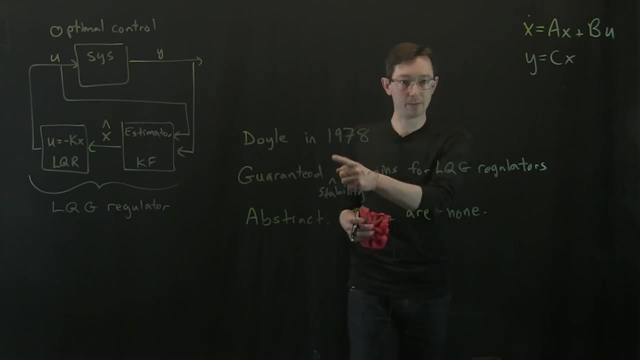 can change the eigenvalues of my estimator, But what this paper is showing is that there's some. the stability of this system does not guarantee that it's robust. It doesn't mean that the system won't blow up if I have some model uncertainty. 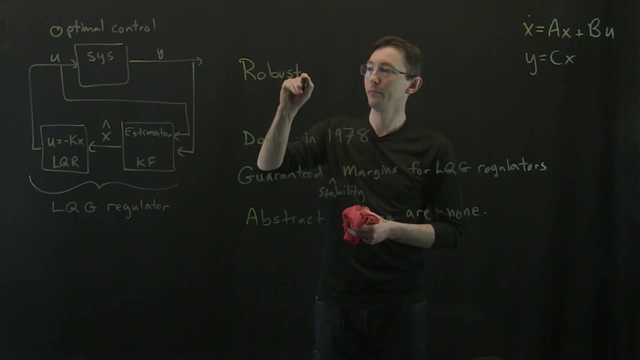 And so there's this new concept of robustness. Okay, And so robustness and performance are now these kind of dual objects. Okay, So the closed loop, eigenvalues of my system and how fast I can estimate, are kind of measures of performance. 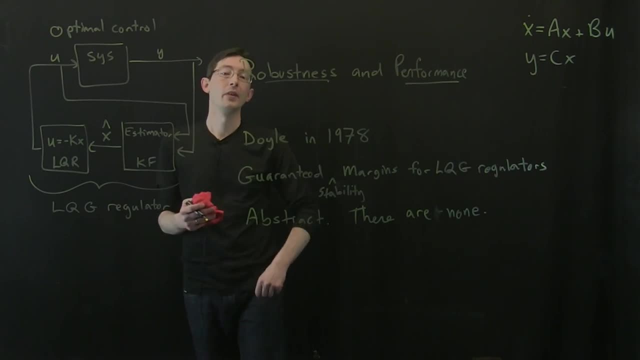 How well does my system perform, How fast does it respond, And robustness is more of a measure of how sensitive is my system to model uncertainties or time delays or disturbances, Things like that. And so in this really fantastic paper, this idea that LQG regulators could have very high 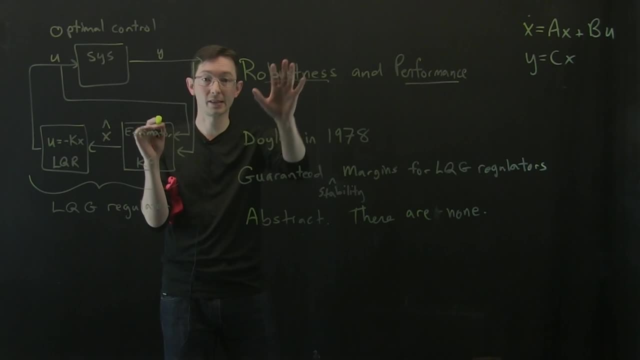 nominal performance, but almost zero robustness really turned the field upside down, and it started this movement towards robust control. Okay, So everything I'm going to tell you about for the next few videos is about robust control. How do we tell if a system is or is not robust to model uncertainty? 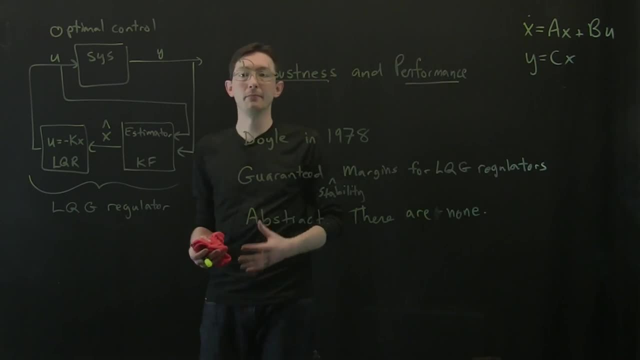 How do we even know what that means? And then, how do we design a system to have high performance and high robustness, And what are the tradeoffs? When can I have both? When can I not have both? Okay, So to jump into this, we're going to need a few new concepts, like the transfer function. 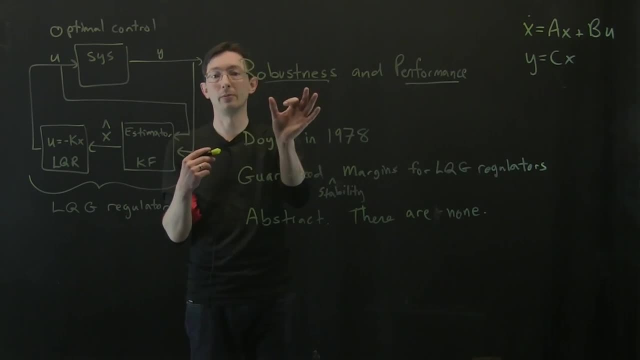 and the frequency domain, because oftentimes performance and robustness are easier to understand in the transfer function or Laplace transform domain. Okay, So that's where things are going. We're going to start figuring out what robustness means, How we can have robust performance, when we can and when we can't, and how to do things. 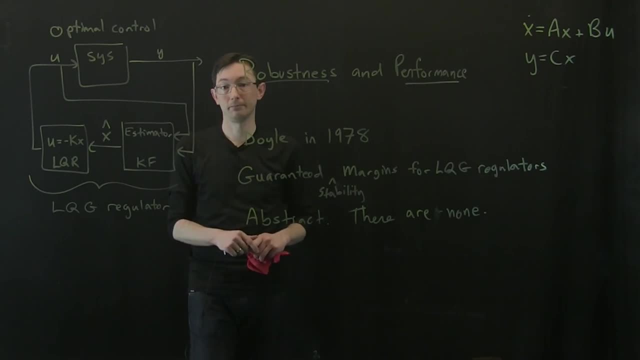 like: fix our LQG regulator to make it more robust. Okay, So that's all coming up and this is going from optimal control to robust control. Thank you,